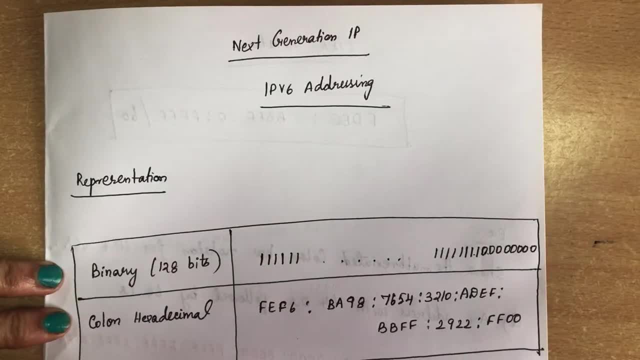 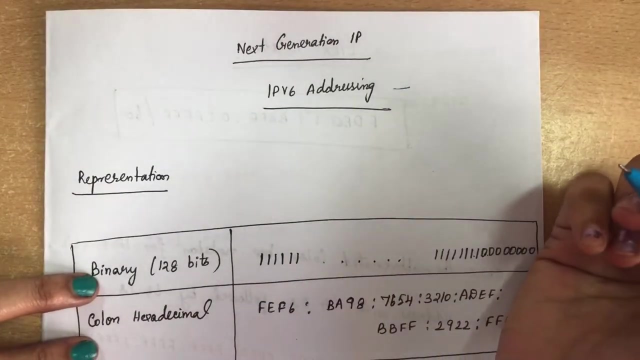 Hello everyone. Today we are going to see a new topic, that is, IP version 6.. IP version 6 addressing, So this comes under third unit of your computer networks, So IP version 6. it is the latest version of internet protocol. So this: using this IP version 6, you can easily identify the devices across internet. Okay, So when you want to identify any device in the internet, you will use a unique addressing. 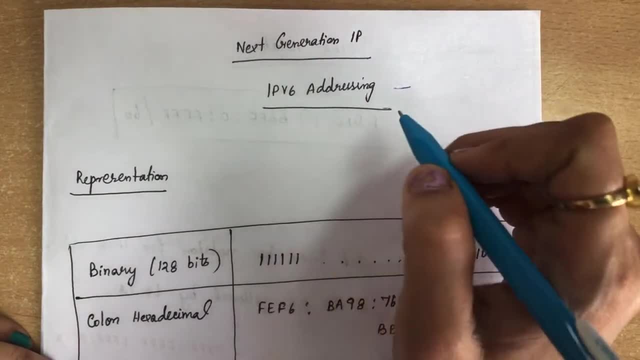 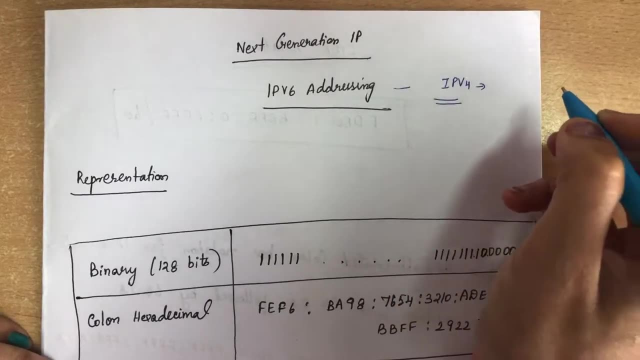 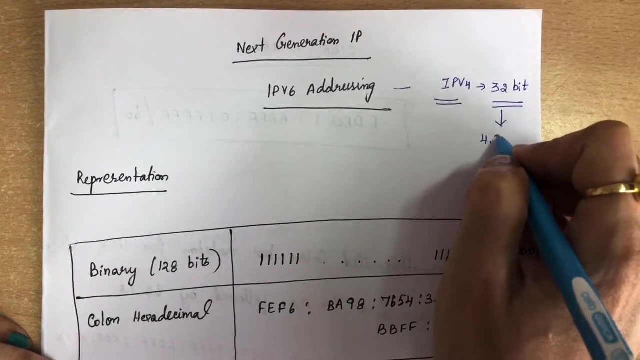 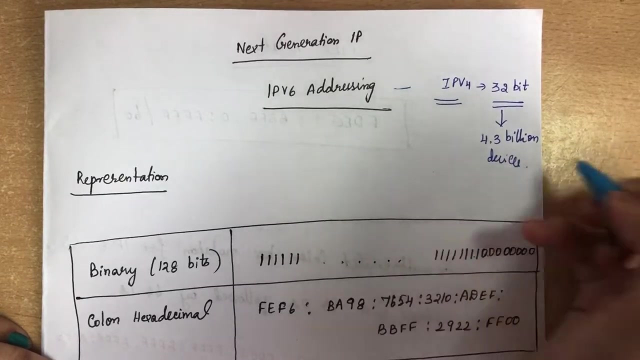 That is called IP version 6 address. Okay, So previously we were using IP version 4.. IP version 4, which we were using across internet to identify the devices, It was 32 bit. It is a 32 bit addressing. Okay, This will support our own 4.3 billion devices. This will support our own 4.3 billion devices, Okay. However, the growth of internet and personal computers, smartphones and now internet of things, 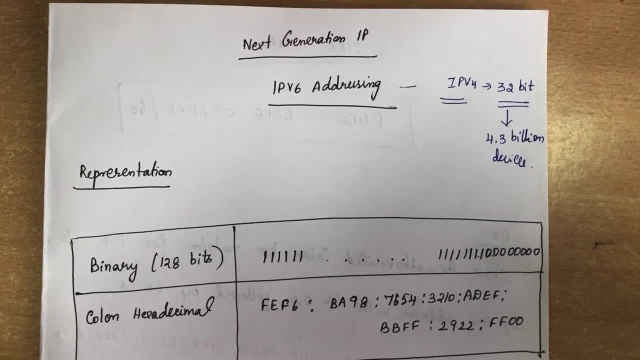 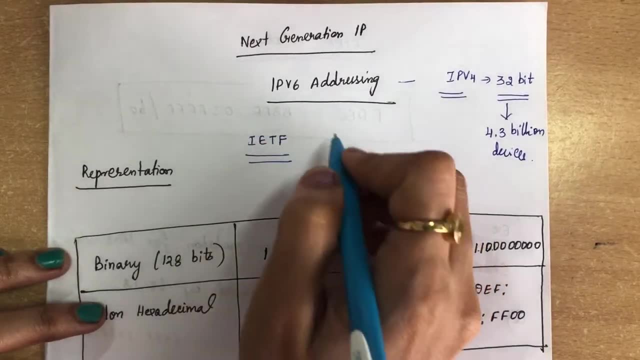 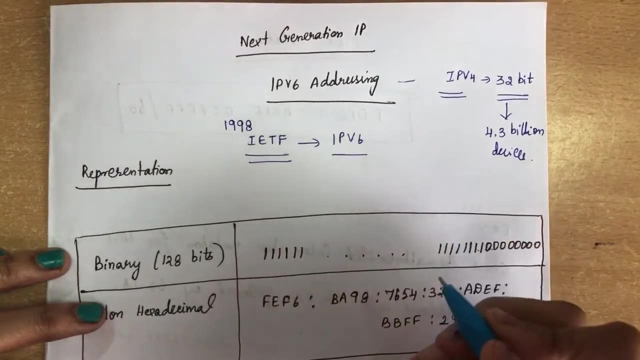 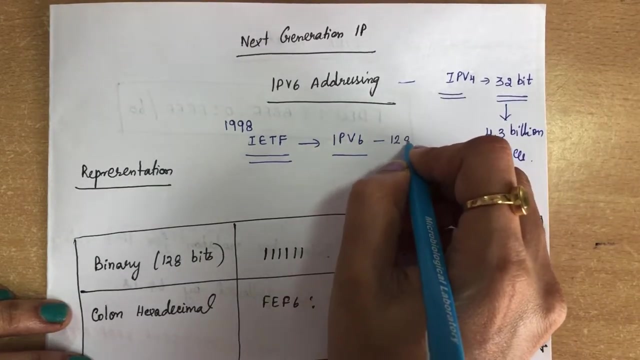 Need more number of addresses. So IETF, that is, internet engineering task force, they have recognized and in the year 1998 they have created a version call addressing new type of addressing call: IP version 6 addressing, where instead of using 32 bit address they have used 128 bit address to support 340 trillion trillion. 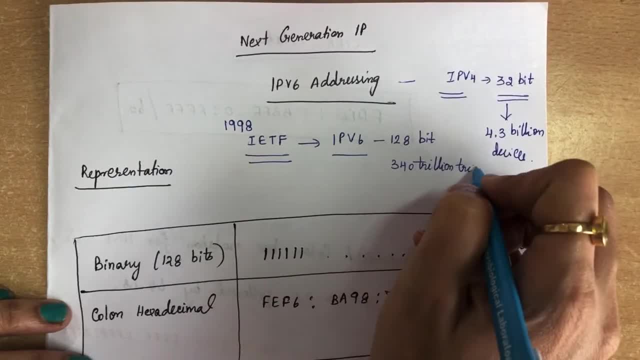 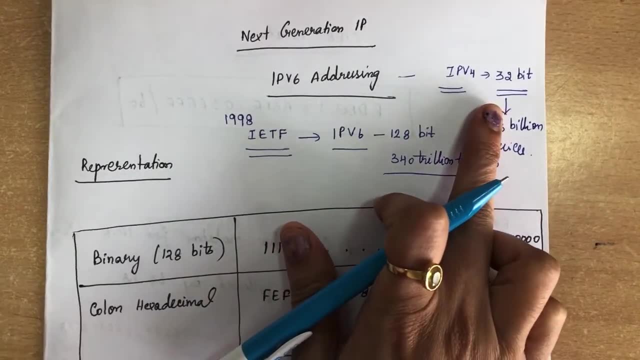 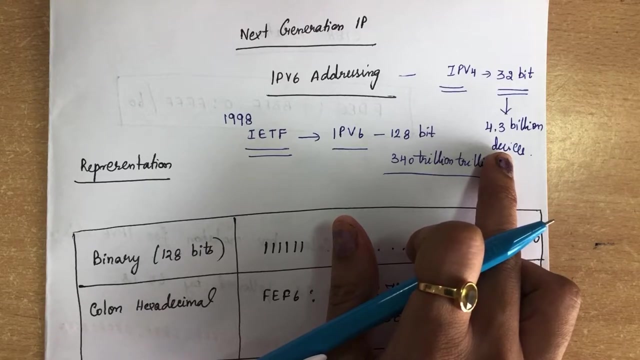 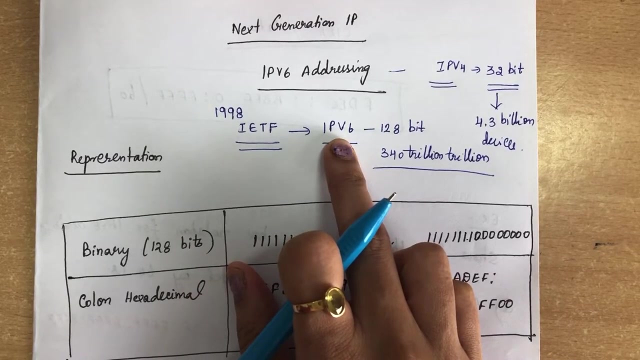 addresses, Okay, Or devices. So IP version 4 it can. it will have only 32 bit address, It will support only 4.3 billion devices. So we need more number of addresses due to the growth of internet. So IETF, in the year 1998 they have created a version, new type of addressing, that is, IP version 6 addressing, which will have 128 bit address, that which can able to support 340 trillion addresses. 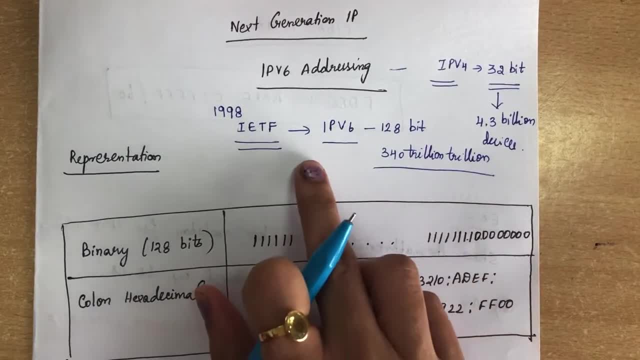 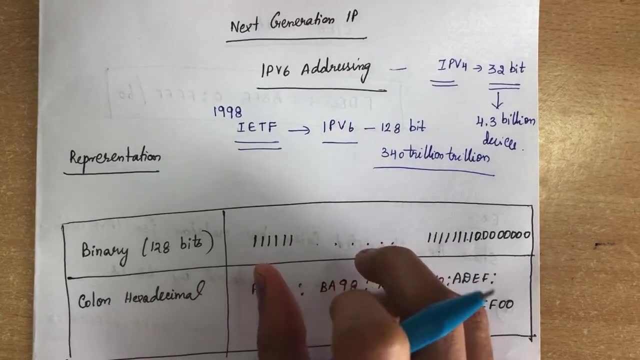 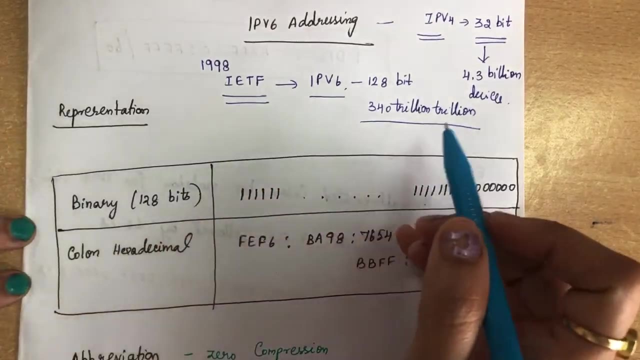 40 trillion trillion devices. that is how this ip version 6 came into existence. so this ip version 4, ip version 6, it will have eight group of four disc hexadecimal digits. they'll be separated by columns. we will see the representation now. so the main reason for migration from ip version 4 to ip: 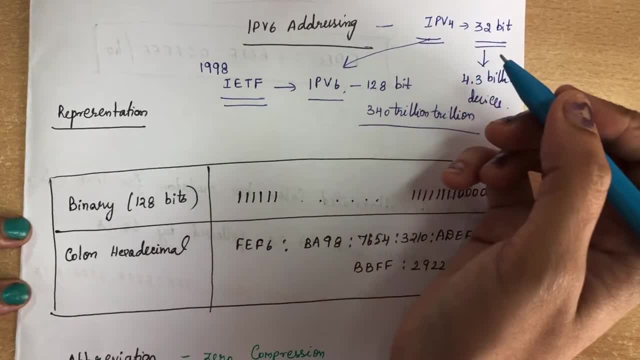 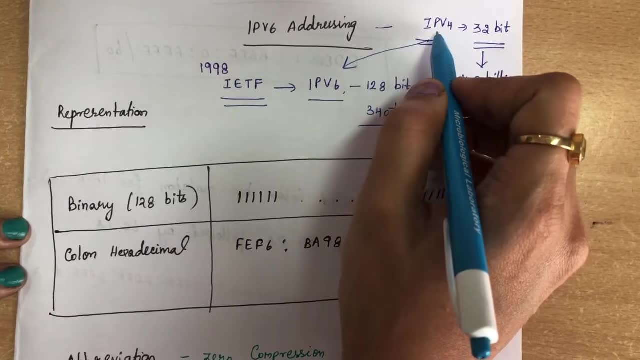 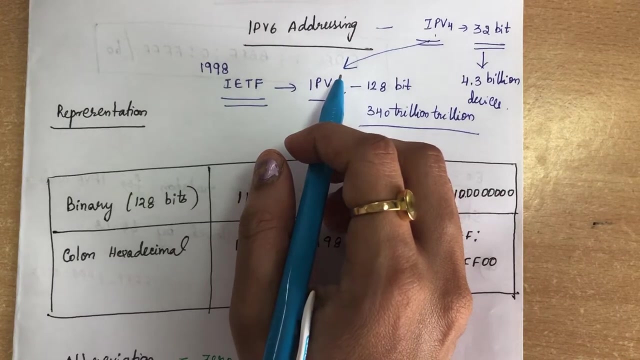 version 6 is the small size of address space in ip version 4 so because of address depletion. so we have converted the version from ip version 4. we have moved from ip version 4 to ip version 6, so this ip version 6 have solved all the problems of address depletion in the future. okay, so how it? 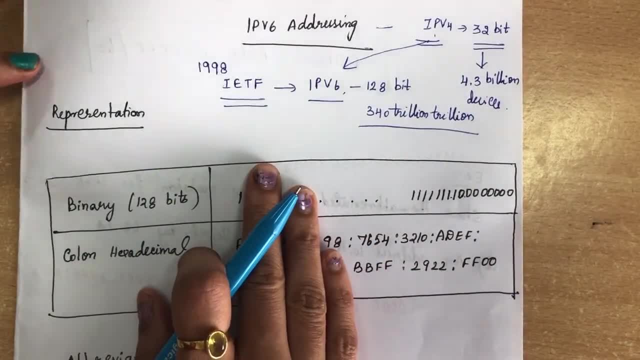 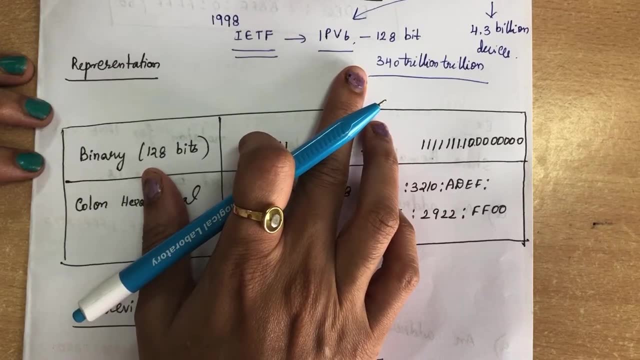 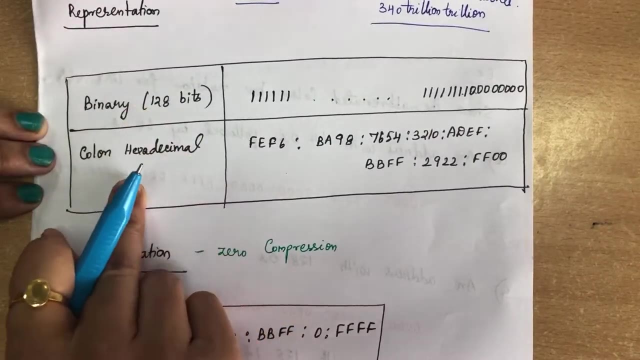 can be represented. usually, computer normally stores the address in binary, but actually this: since this ip version 6 is 128 bits, it is cannot be easily handled by humans. so several notations have been proposed to represent this ip version 6. so the two notations have been represented over here. the first one is binary representation, where 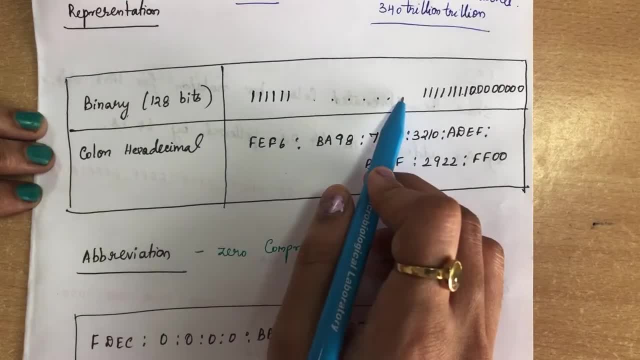 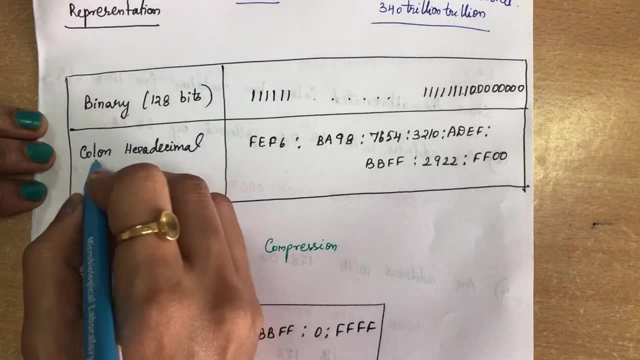 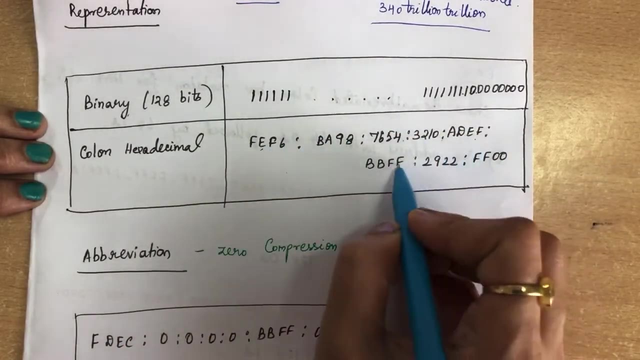 you will be representing the 128 bits in binary numbers, in either zeros or ones. second notation is hexadecimal notation, where it is called this or otherwise, colon hexadecimal. here we are going to divide this address into eight sections, so you can see there are eight sections over here. 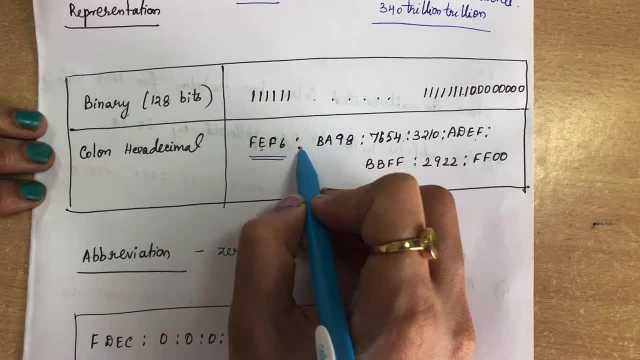 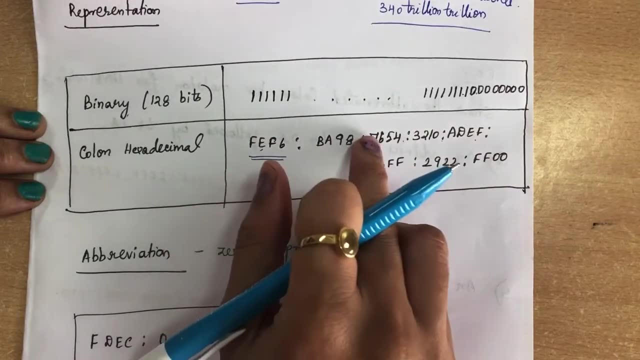 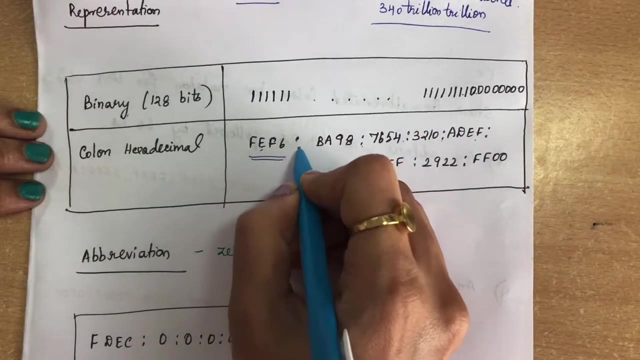 each made with four hexadecimal digits and they are separated by columns, so you will be dividing the entire 128 bits into eight sections. so you can see eight sections over here and they have been represented each with four hexadecimal digits and they are separated by columns, so you 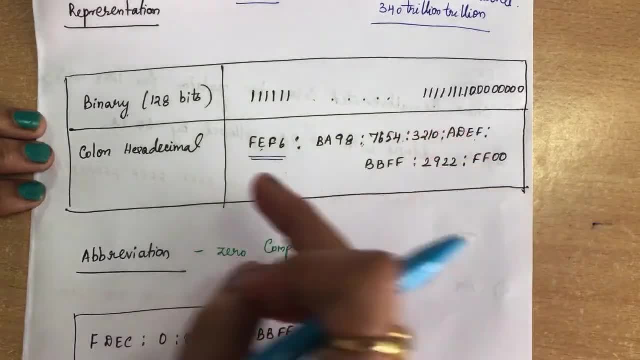 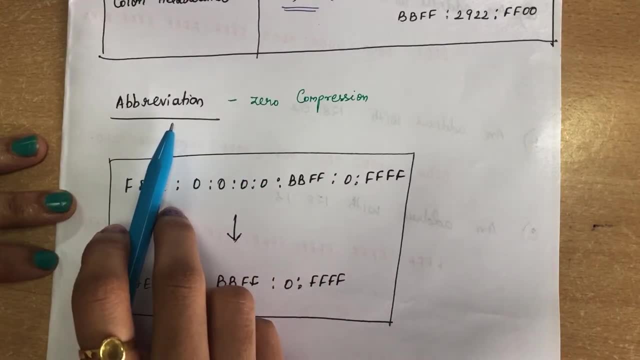 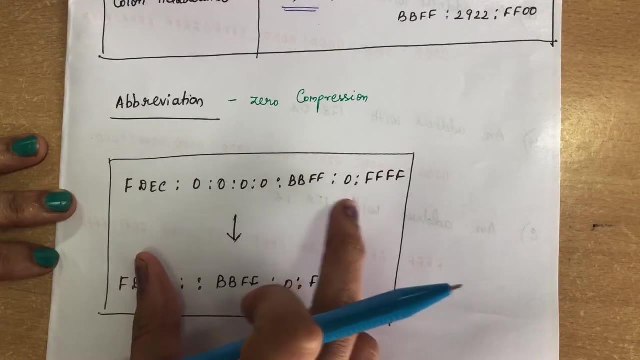 can? you can represent this like this. okay, this is how you can represent your ip version 6 notation. next, we will see the abbreviation in ip version 6. so in when you are representing this ip version 6, you can see the number of digits as well as the number of hexadecimal digits. so this is the. 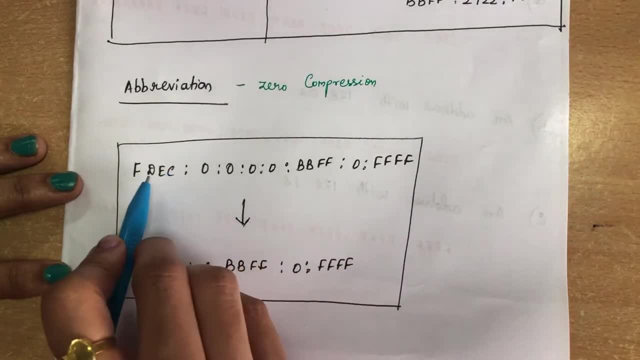 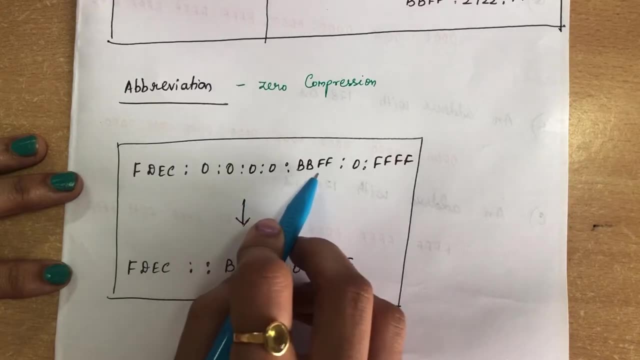 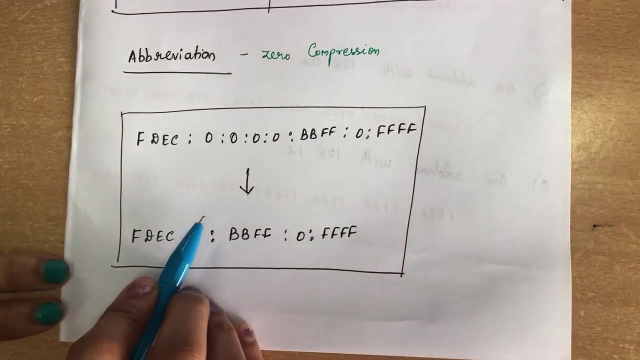 number of hexadecimal digits of the ip, version 6. so let's see what we can do here so we can abbreviate this address. so if you are having the ip address like this, fdec, colon 40, so i have represented only 0 over here, colon 0, colon 0, colon 0 and again one more hexadecimal digits and colon. 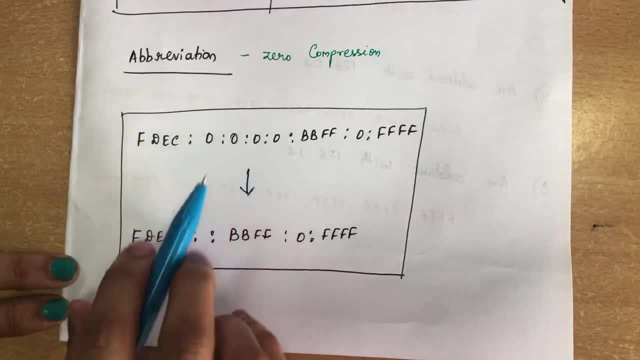 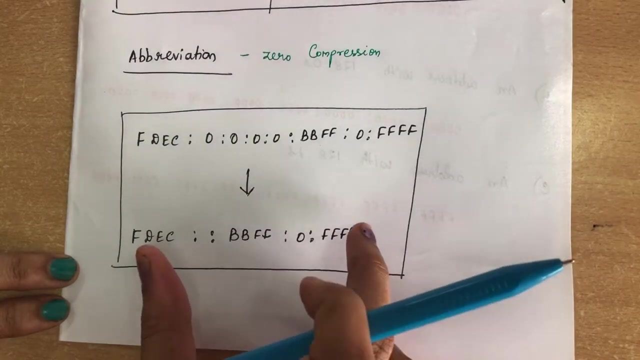 fff. so i can represent this. i can shorten this ip address like this: fdec, colon, colon, so all the zeros in double colon, and then BBFF, colon, 0, colon, FFFF, So this is called zero compression. So here we are going to reduce the number of digits in your IP address by representing like this: So we are. 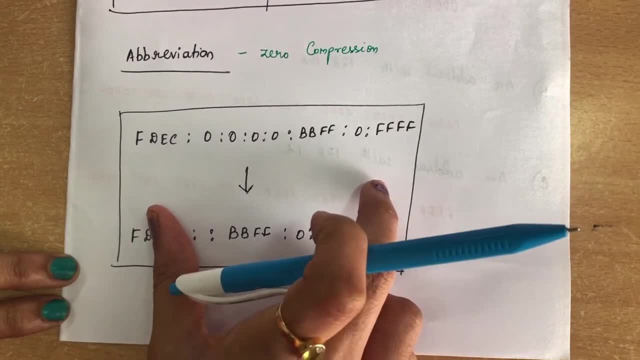 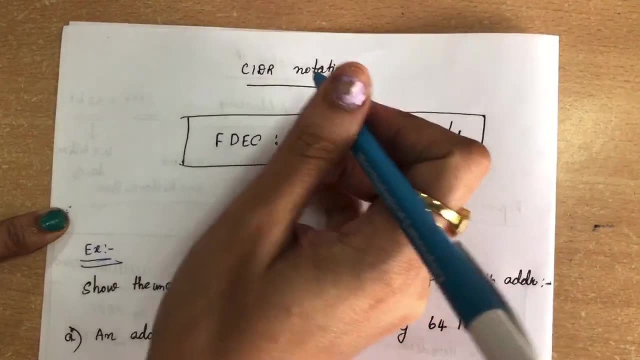 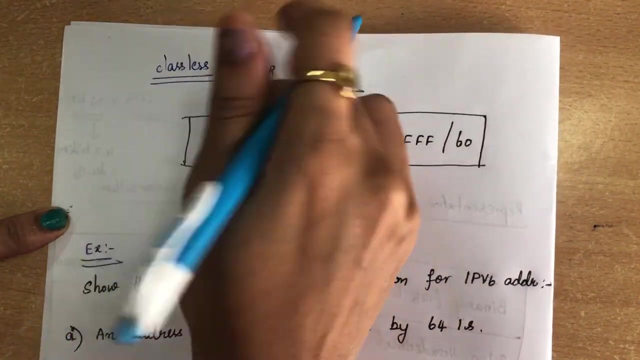 going to compress the zeros over here in your actual IP address. This format is called zero compression. We will see how IP version 6 is represented in classless addressing. In classless addressing it is represented in a notation called CIDR. It is nothing but classless. We have already 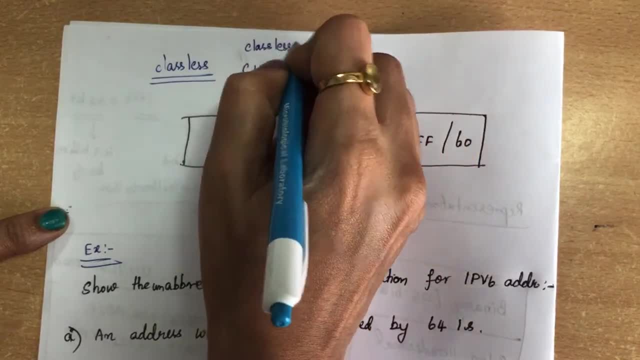 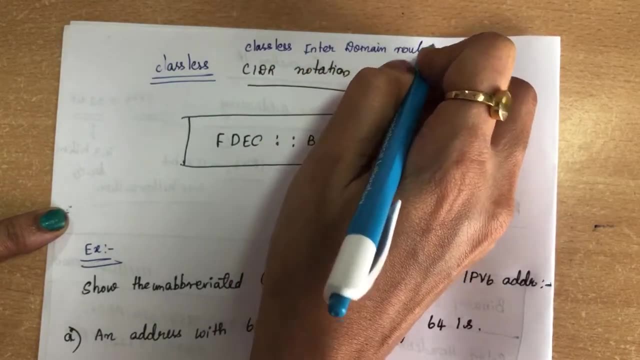 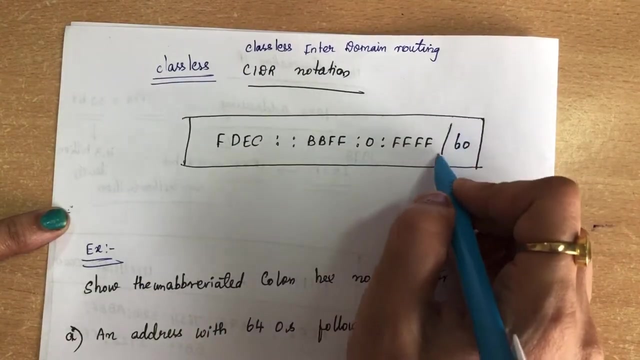 seen when we have discussed in IP version 4.. It is classless, inter domain routing, Inter domain routing. So when we want to represent in classful addressing we can represent the simple IP address. When we want to represent in classless addressing we should use a slash notation and the number of 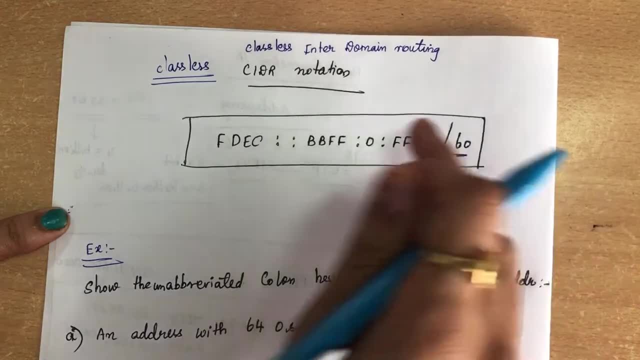 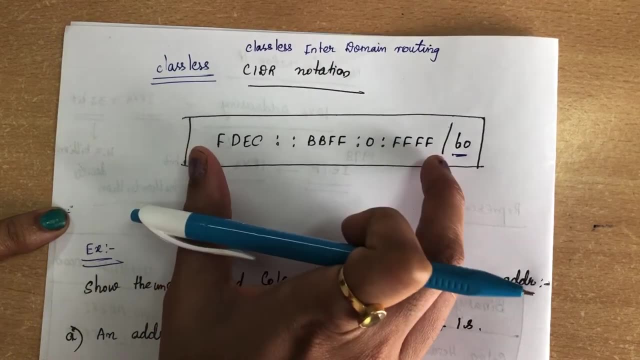 bits that can be considered as prefix can be given over here. So this is how we are going to represent in classless addressing. This is how we will represent this IP address in classless notation, The IP address of 128 bits and which can also be represented in hexadecimal format over here: slash, and here the number of. 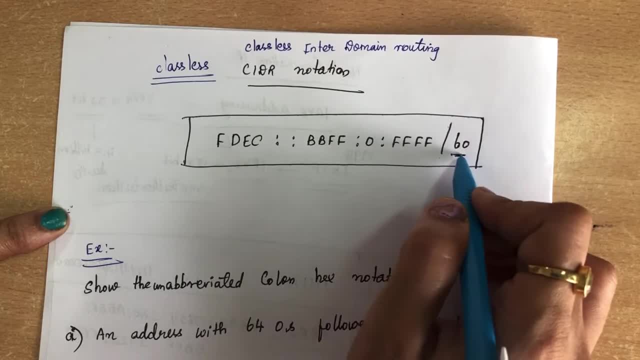 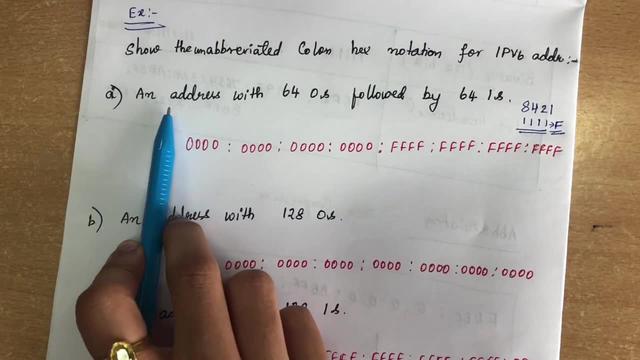 bits represent how many number of bits we have considered as a prefix. This is your CIDR notation. Next we will see some examples. So here they have given you some address and you have to convert that into a notation called IP version 6 address notation. So the first one is an. 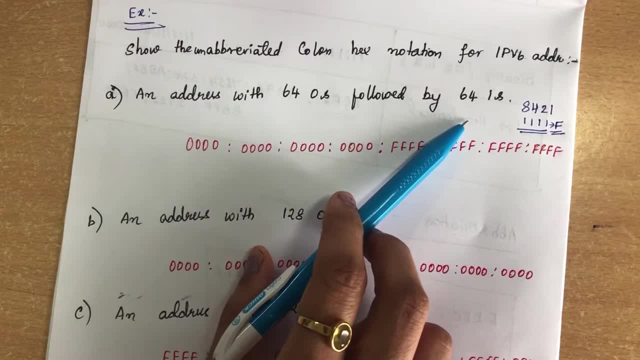 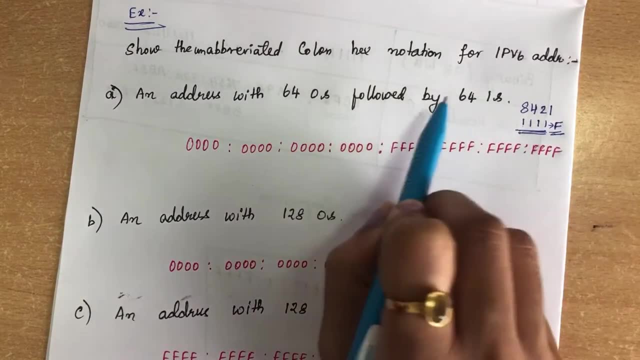 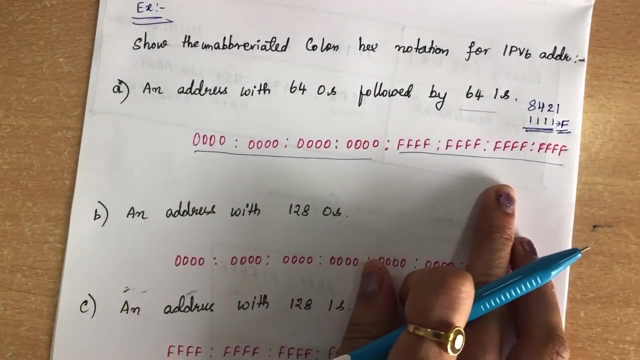 address with 64 zeros followed by 64 ones. So when we represent in 8421 format, when it is all one, it is nothing but F. That is why 64 zeros are represented like this and 64 ones are represented like this. So this is the IP version 6 format for this particular question. Suppose if 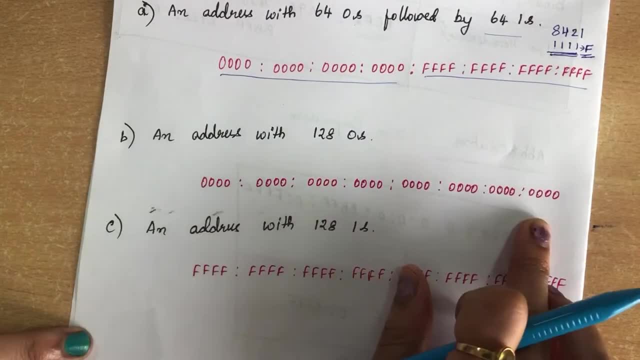 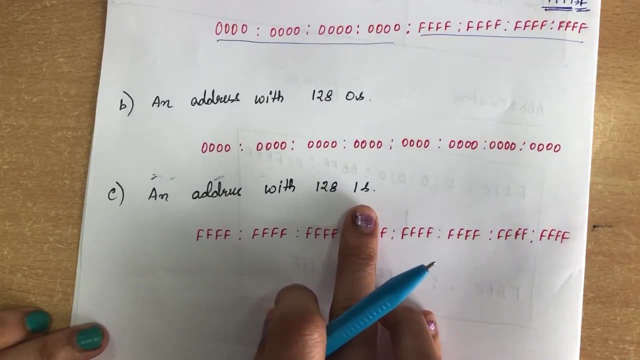 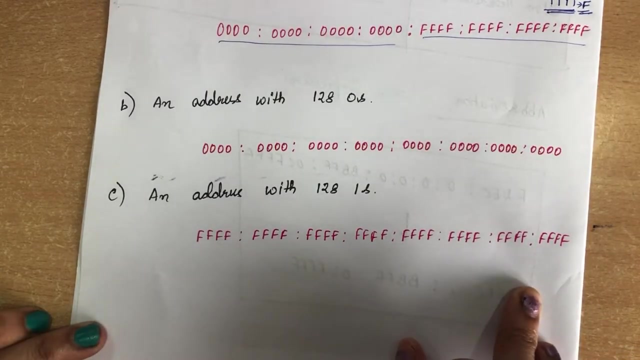 they are asking an address with 128 zeros, all numbers will be represented in zeros When they have given all the numbers in by one, 128 ones. when you want to convert into hexadecimal format, all everything that hexadecimal digits will be will be represented in F. So this is how you have to convert the binary form into hexadecimal. 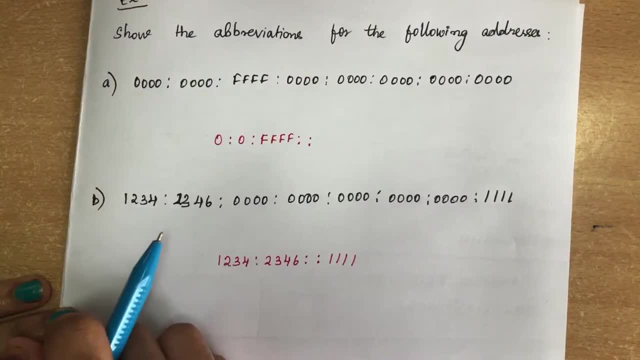 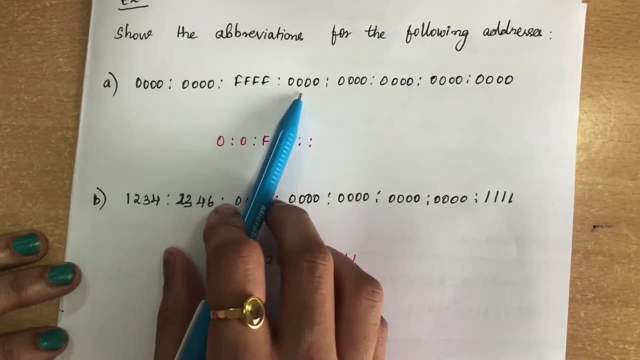 form. You understood this. See some abbreviations for the following address. Suppose: if they have given four zeros colon, four zeros colon and then F, F, F, colon, zeros, followed by zeros, zeros, zeros. So this can be short, we can shorten this IP address and we can represent. 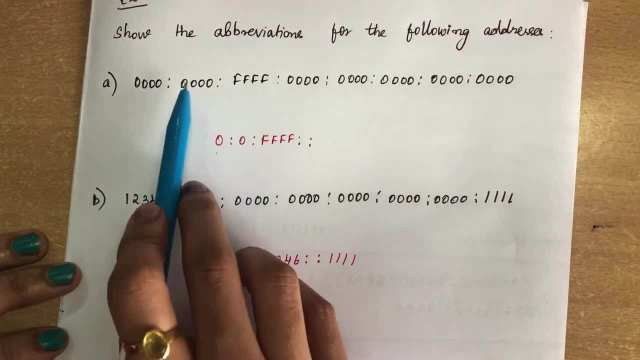 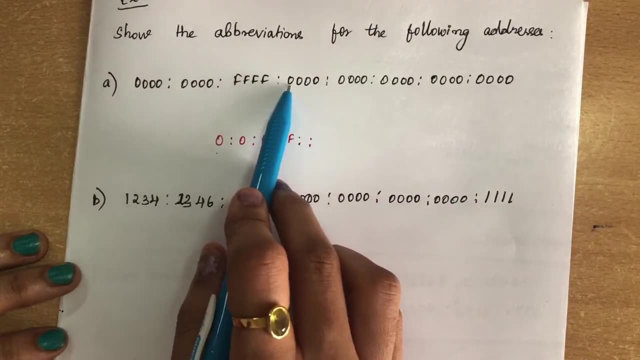 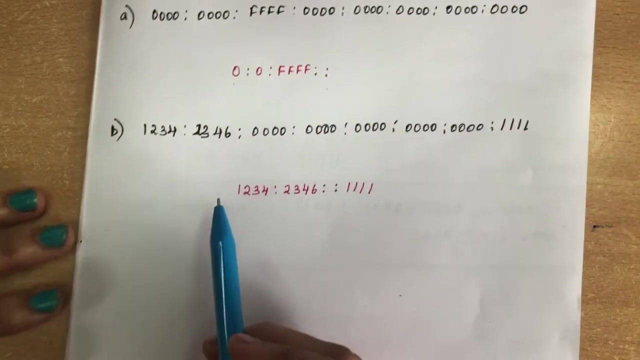 it like this: So four zeros can be represented by zero colon and these four zeros can be represented by zero. again colon: F, F, F, then all, then it is followed only by zero. So we can represent it by double column. So this is how. what we can do is we can shorten your IP address. The next one is: 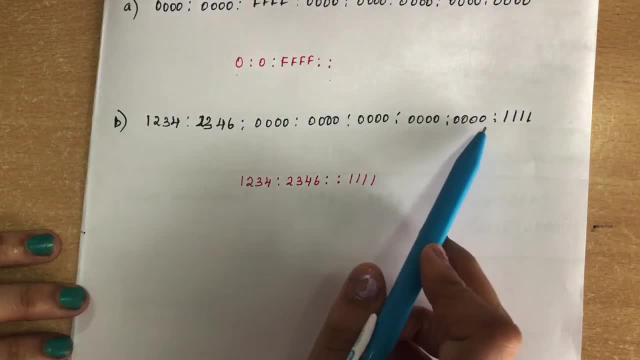 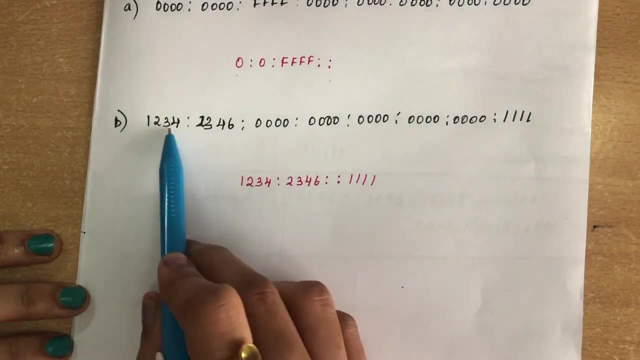 1234, colon 2346. then you have zeros and again, lastly, it is- it ended with 1111.. So when you are going to shorten this, you will get 1234, colon 2346. So all your zeros can be represented as colon, colon. At last we have 1111.. This is how. 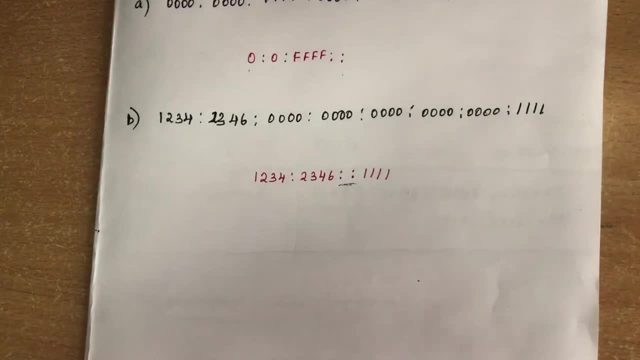 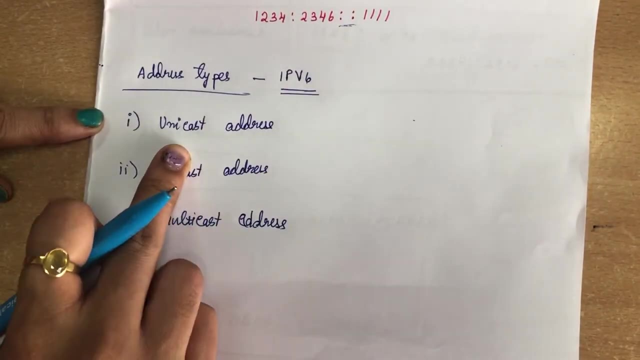 it will be shortened like: this is how you can shorten your IP address. Okay, See the addressing types in IP version 6.. Okay, There are three. it will support three addressing type. One is unicast address, Second one is anycast address and third one is multicast address. Coming to unicast address, 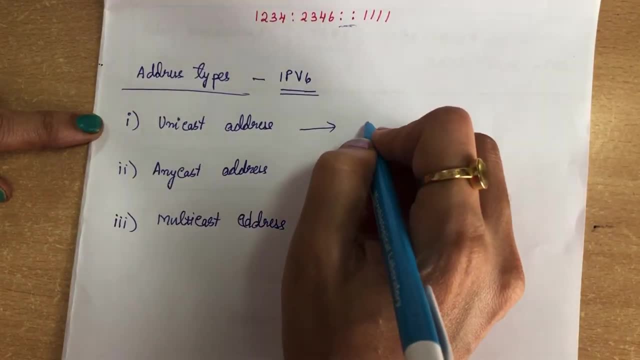 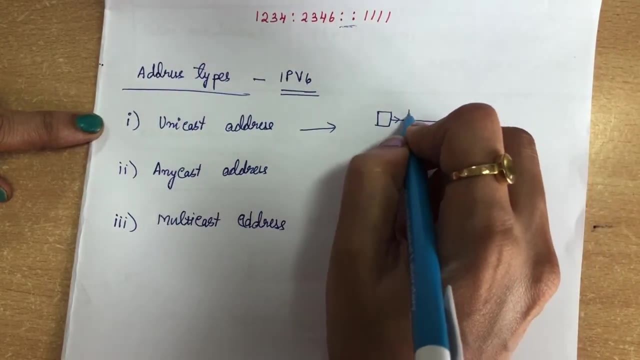 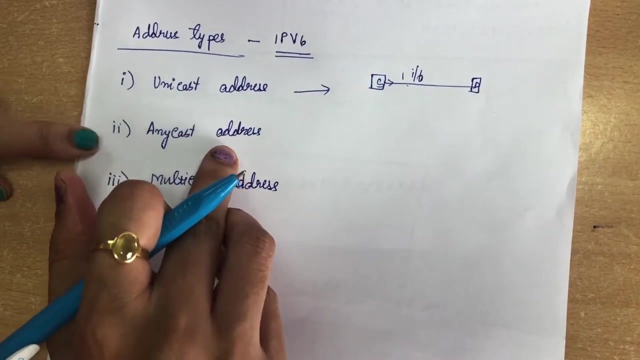 so here the packet will be sent to the intended receiver, So using one single interface. if you source and you have a destination, so the packet will be sent through one interface and it will be sent from source to destination. So that is not a problem in case of unicast, In case of anycast. 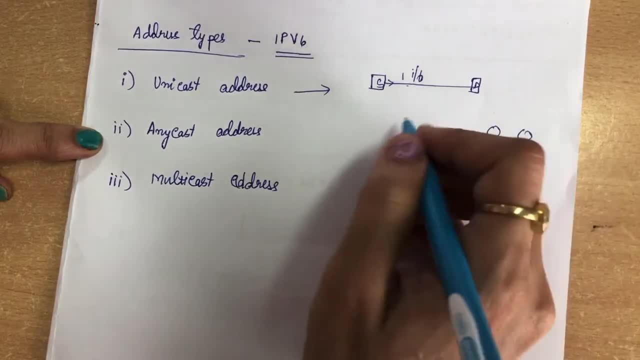 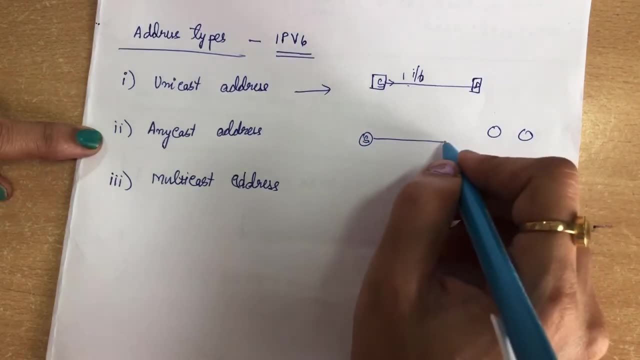 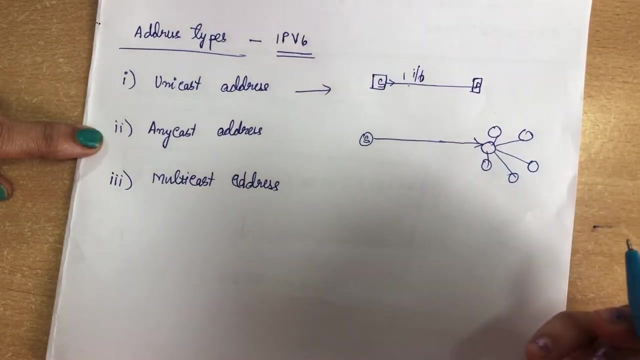 addressing. suppose you have a group of computers, Okay, And here you have a sender. So what happens is this packet will be delivered to any one of the member. Okay, There will be any one of the member. the packet will be delivered from there. it will be sent to all the groups of the members. 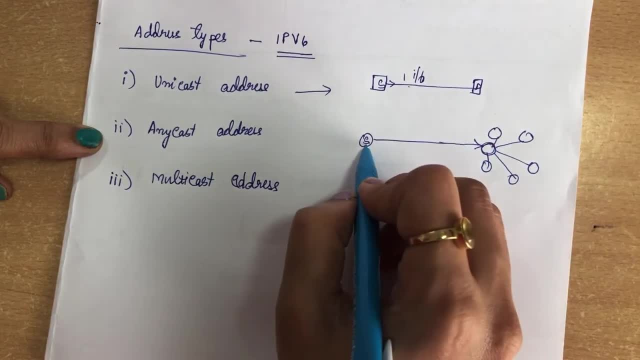 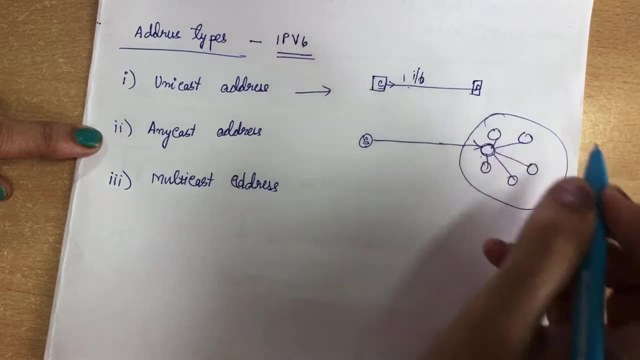 So there will be one single point of contact which will be communicating with the sender and it will be receiving the packet that is anycast address. So here it will: all the addresses, all the computers, they will share a single address. Okay, Single address and only one packet will. 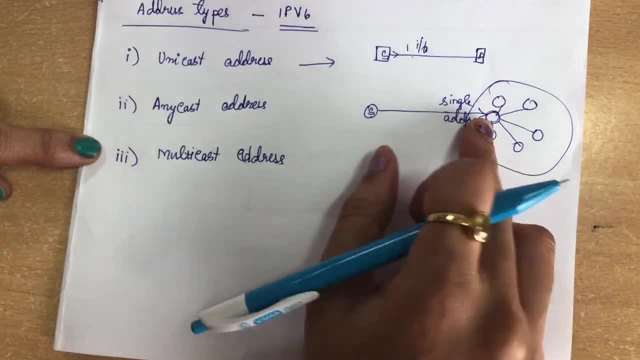 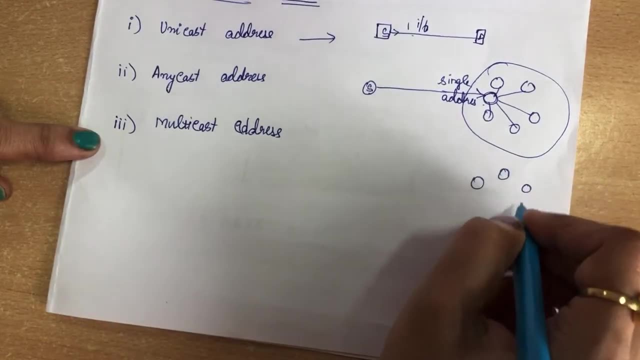 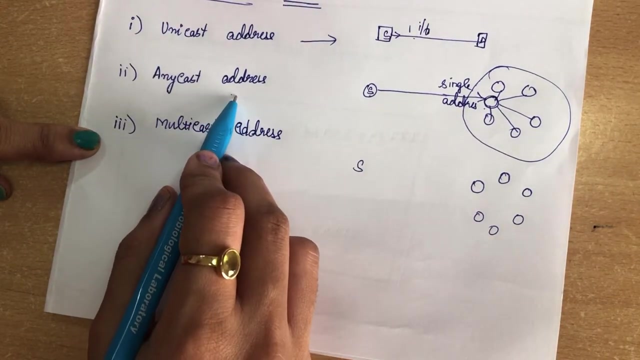 be sent to the one, the most reachable node in that particular network, that is, anycast address Coming to multicast address, here also you have group of computers. but the difference between this anycast address and as well as multicast addresses? in anycast address, only one copy of the packet will be sent. One copy of packet will be sent to any one of the member. 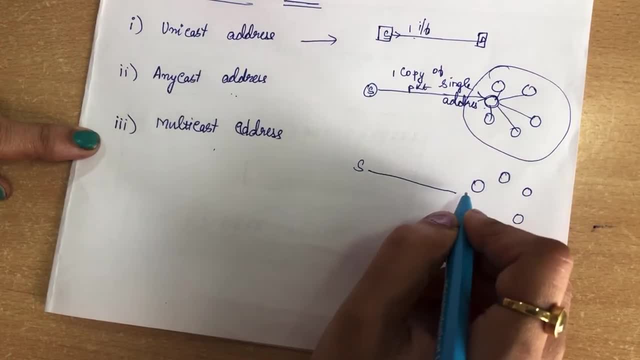 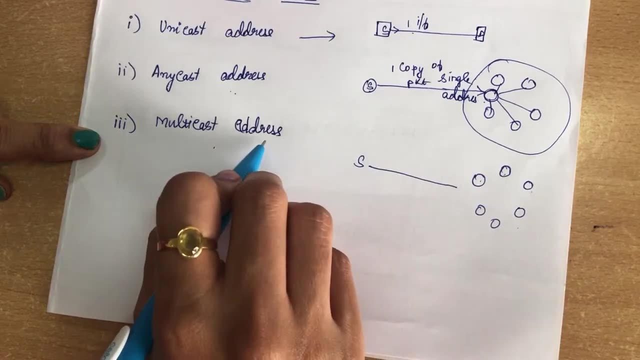 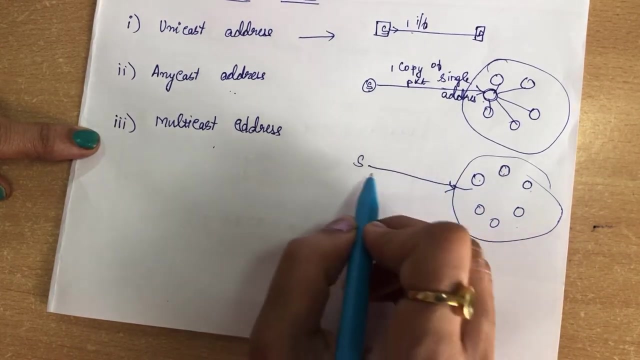 inside the group, But here there will be each. that is like here: each member of the group will receive one, one copy. So that is the difference between multicast address. So here what happens is here also, it will be sent the group. So once if you are going to send a packet from the source, 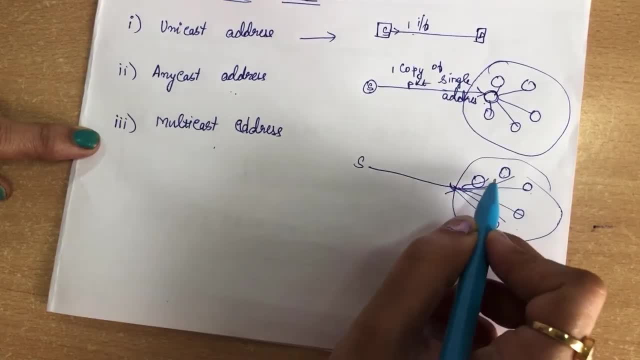 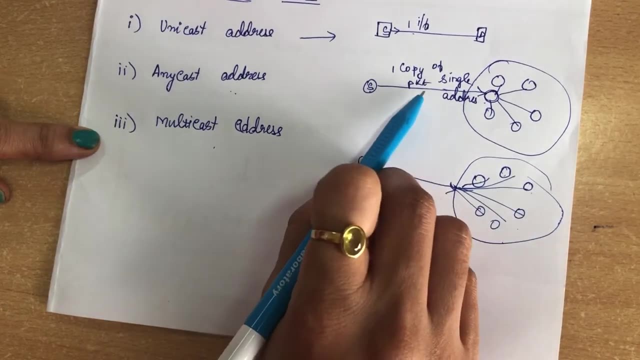 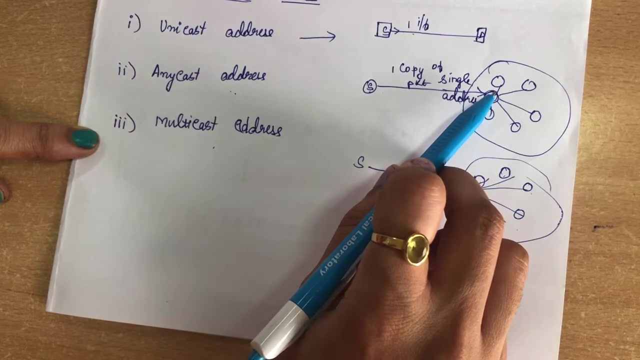 it will be sent to all the persons inside the group, But every group of the member will get the different will get the duplicate copies of the packet, But here only one packet will be sent out from the sender and it will be sent to the most reachable node in the group. 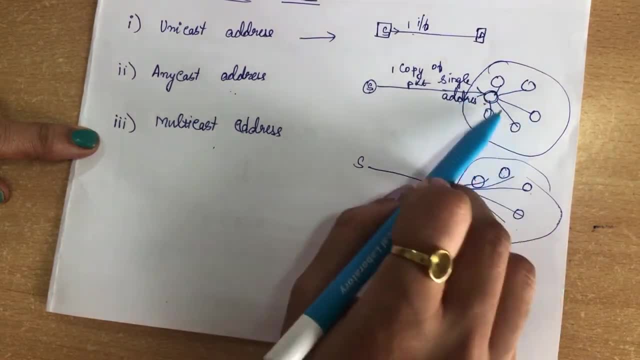 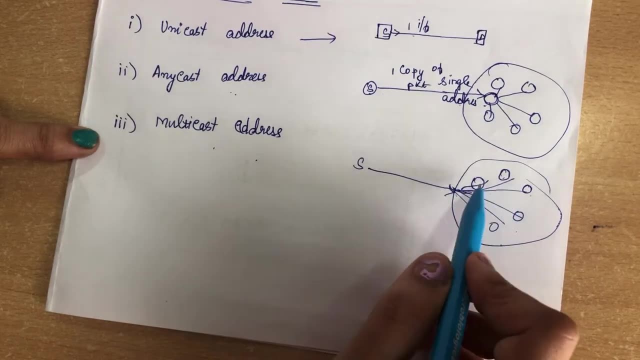 And from that that packet will be sent to all the groups in the members. But here in multicasting what happens is a sender will send a packet, but it will be sent. that packet will be sent to all the persons inside All the group of the members, all the group of the members inside the group. So it receives. 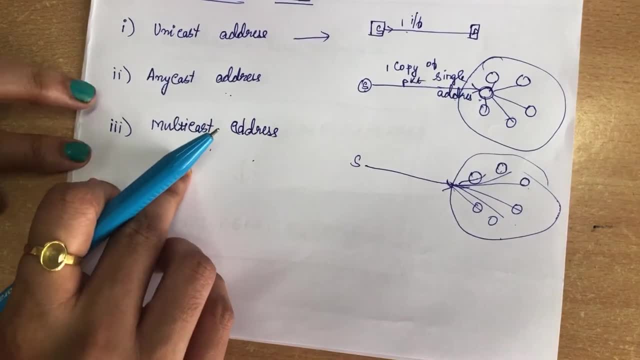 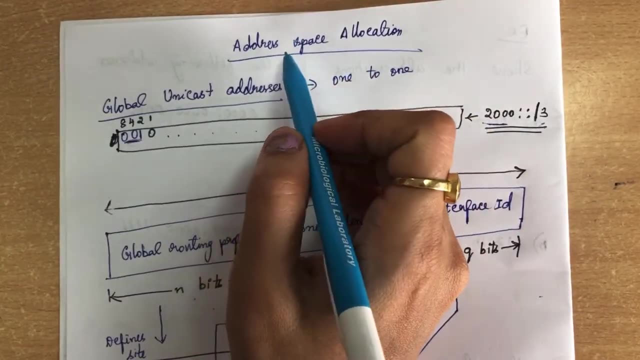 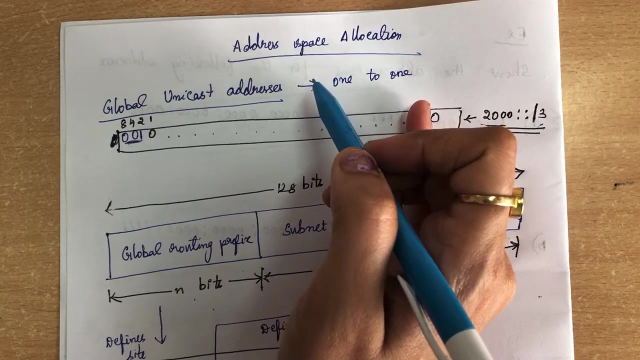 every member of the group, it will receive a copy. That is the difference between multicast address and anycast address. You all understood this Address space. Like the address space of IP version 4, IP version 6 is also divided into several blocks and with varying size, and each block is allocated for specific purpose. 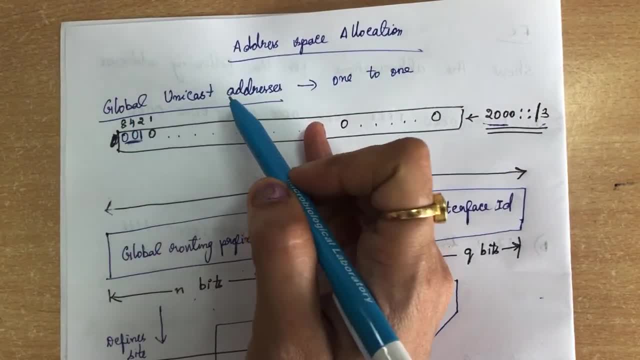 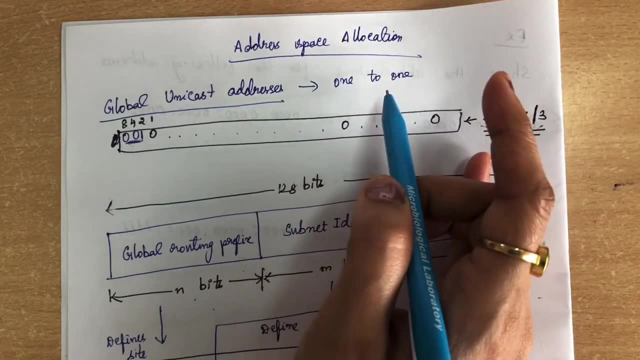 First we will see the one type of block, that is, global unicast address. So what do you mean by global unicast address over here is it is used for one to one communication between any two host inside the network. So if you want to do any one to one communication, 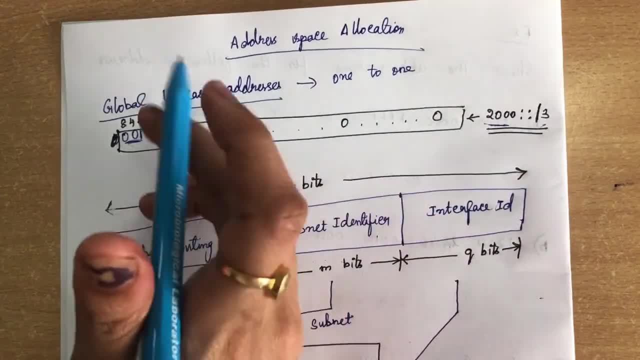 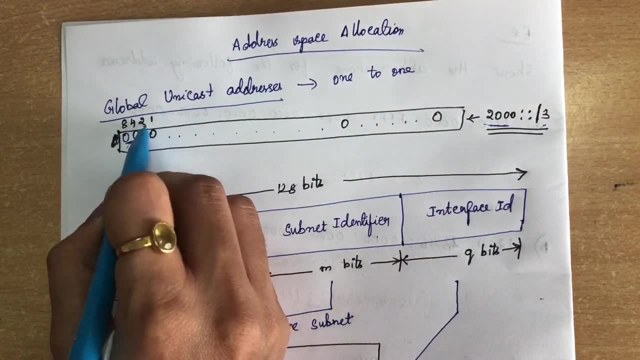 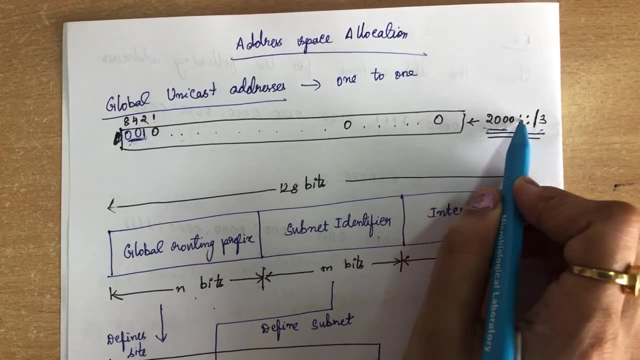 inside the internet you can use this particular address. So the first three bits it will be 001, that is 8. if you are represented in 8421 format it is nothing but 2.. So in all zeros it will start with this number. So we can represent it in hexadecimal format: 2000 colon. colon slash 3.. 3 bits is nothing but 2.. So if you want to do any one to one communication between any two host inside the network, So if you want to do any one to one communication between any two host inside the network, So you can represent it in hexadecimal format. 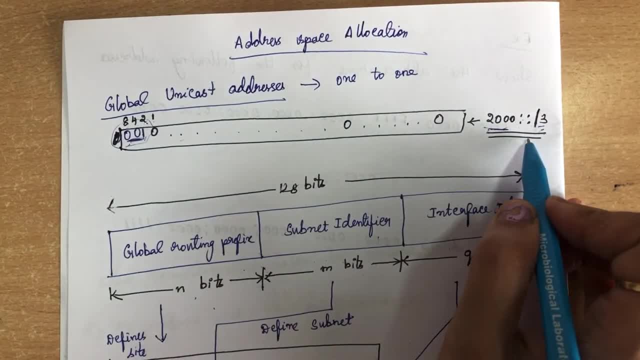 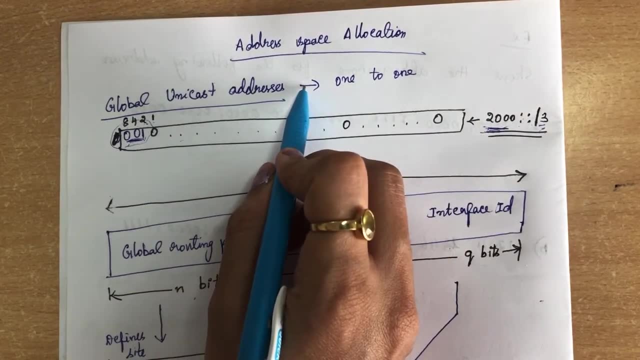 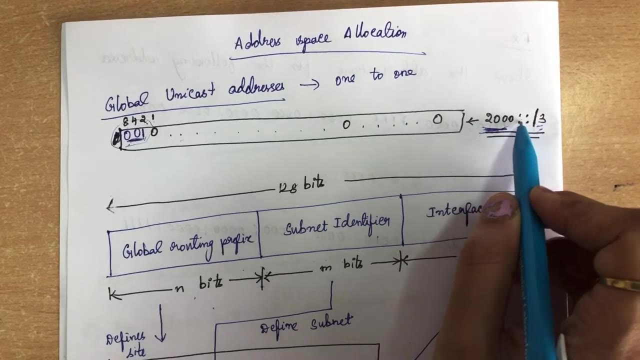 3000 colon, slash 3.. So any block which is starting with this, any host which is starting with this 2000, can use this unicast communication. So all the host will have starting address like this 2000 colon, some any numbers you can have over here. Ok, So this is represented. 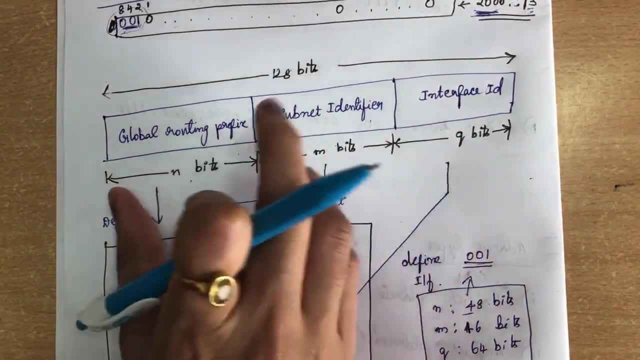 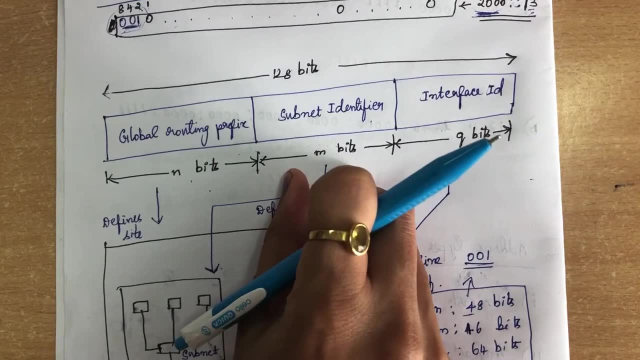 as like this: So here you have the 128 bits. it can be divided into three blocks: One is prefix, is difficile, which contains the prefix, and one is unicast. So you can see that it n bits, subnet identifier, which contains m bits, and interface, which contains q bits. this global. 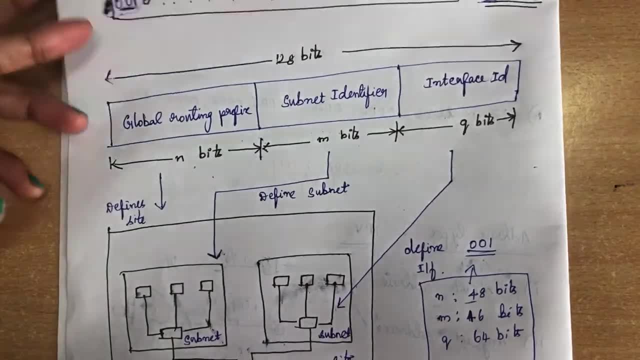 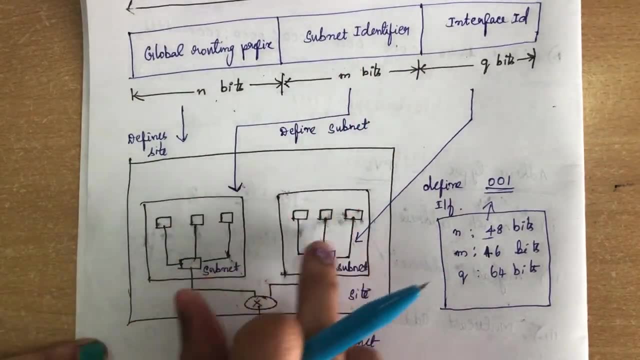 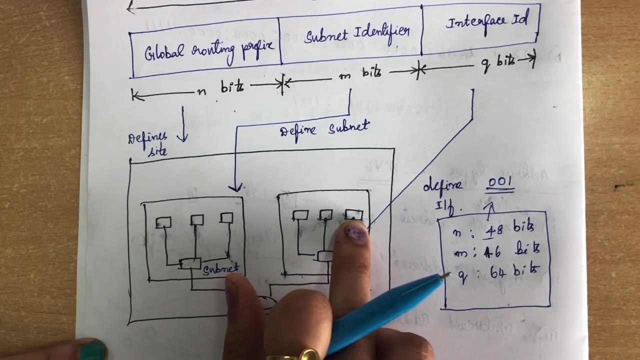 routing prefix is used to identify the site of your internet, in which site your net system has been connected, and subnet is used to identify your subnets inside your internet and interface is used to connect is used to identify the device or interface in the inside your subnet. okay, this. 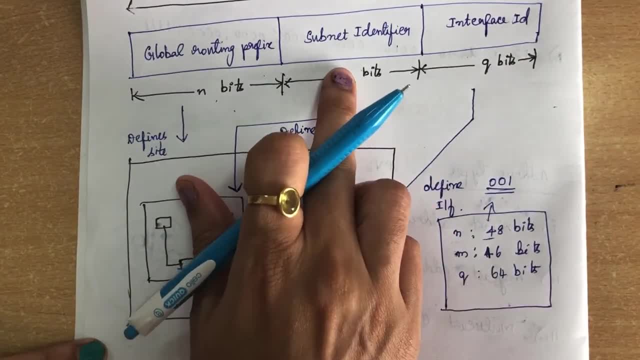 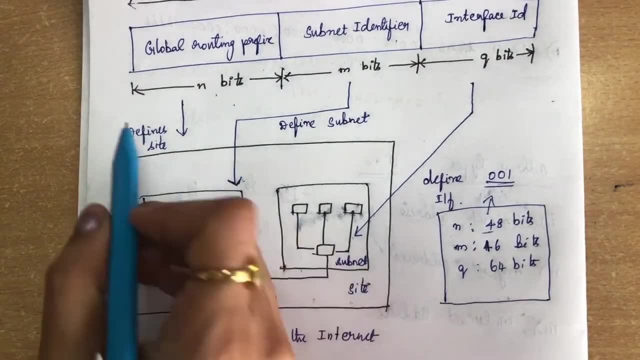 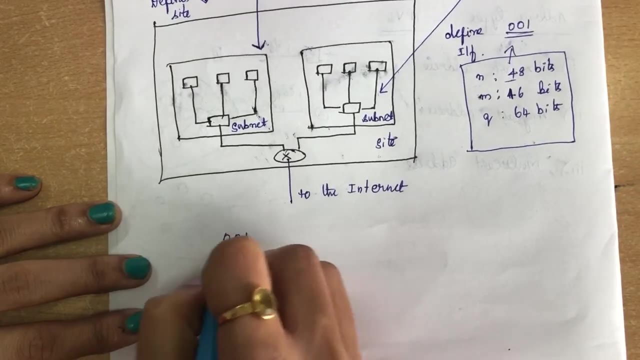 global routing prefix will have 48 bits and the subnet may contain 46 bits and this interface can contain this 64 bits. okay, so the first three bits over here in case of global unicast addressing, is 001. the first three bits is 001. okay, so, totally, you have 10 bits, that is 48 bits are there in? 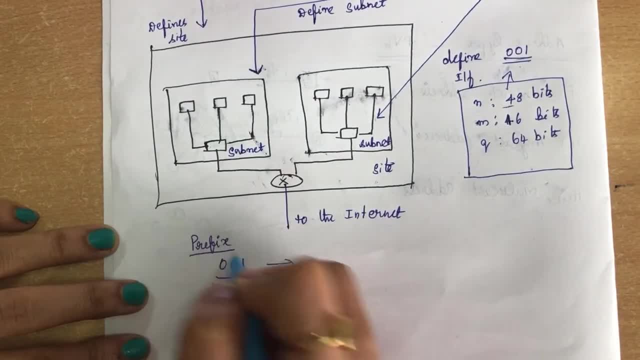 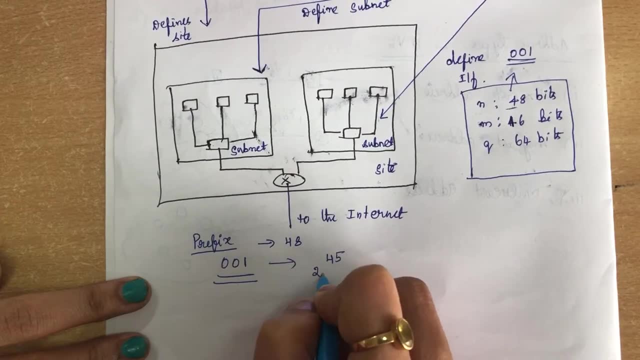 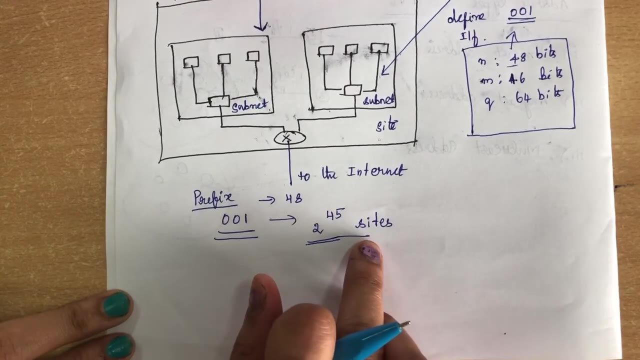 your prefix. in your prefix, global routing prefix, you have 48 bits, among which three bits have been is fixed also already. so you have only two to the power of 45. you can able to allocate to a private organization two power 45 sites: a private organization or an isp- okay, you, this is no. 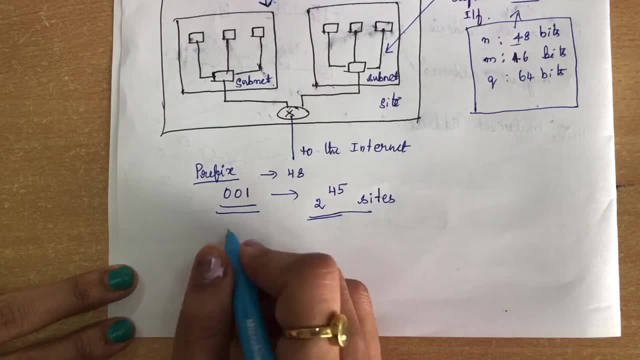 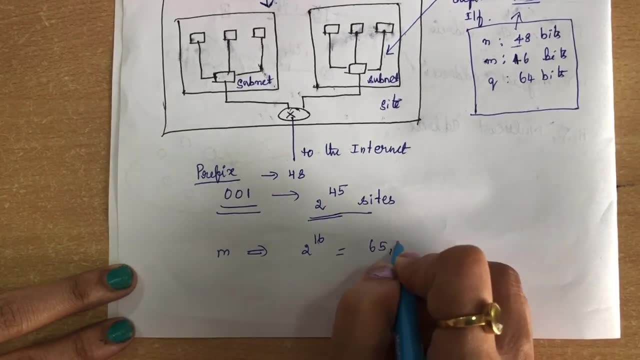 this is more than enough to allocate, okay. next, coming to this: m bits. m bits, if you take it, is already two power 16. that is nothing but 65 536 subnets you can able to allocate. this addresses can be allocated to. it may be allocated to. 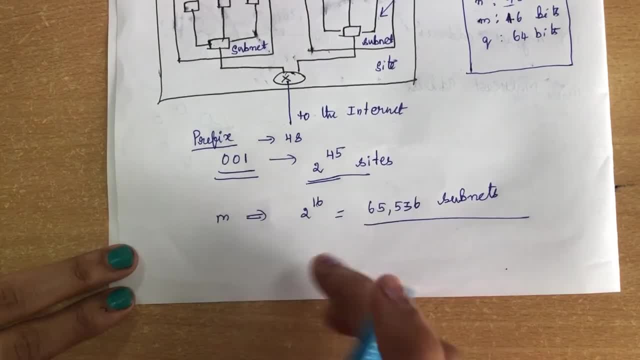 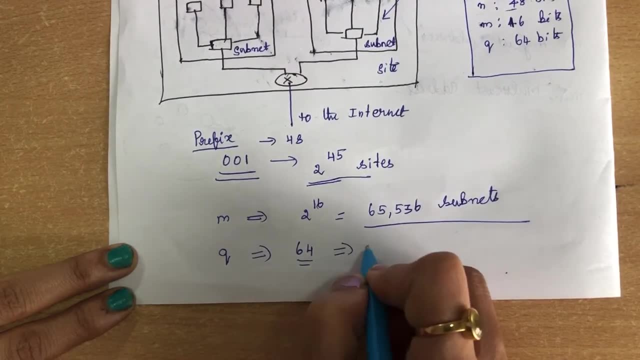 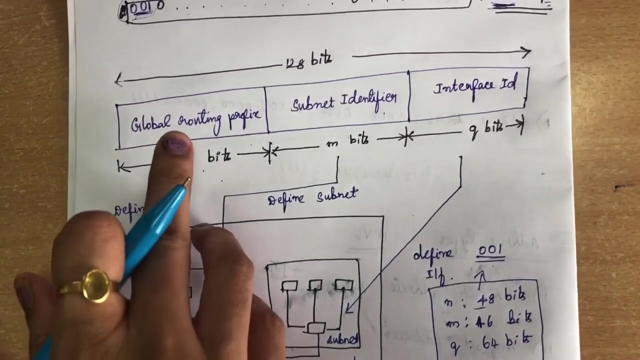 6500536 subnets, which is more than enough, i think so. next, coming to this interface bits, that is cubits it is. you have 64 bits over here, so it is two power 64, which is also more than enough to allocate the addresses. so here the global, this global unicast address is, is been divided into: 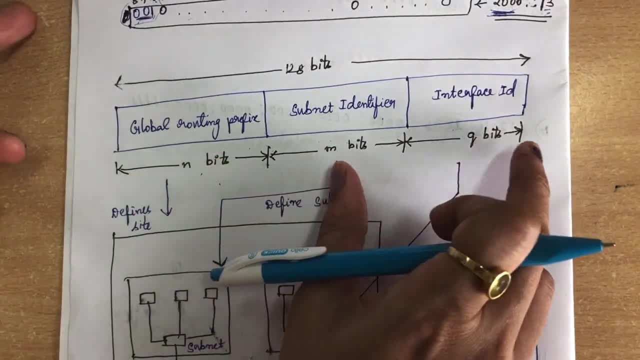 three blocks. one is used for prefix, second one is subnet and third is interface. this prefix already first three bits fixed and you can allocate however your Sabotage refreezer bin programs is unique and often have them fixed. examples also: you will findabeios. also may be other industries which are launching Soon coz of my point that robots also. I use b野 illustrations softwares To see what is my point. there are KК-合άλ. If we want to change software, feel free to touch bar Lit 2 and A. 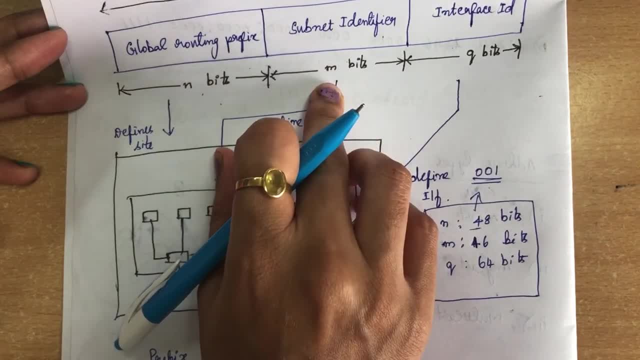 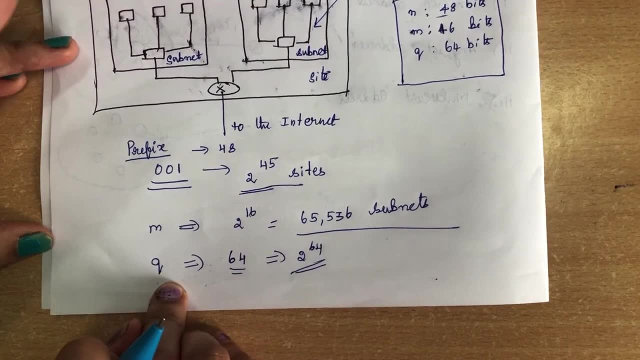 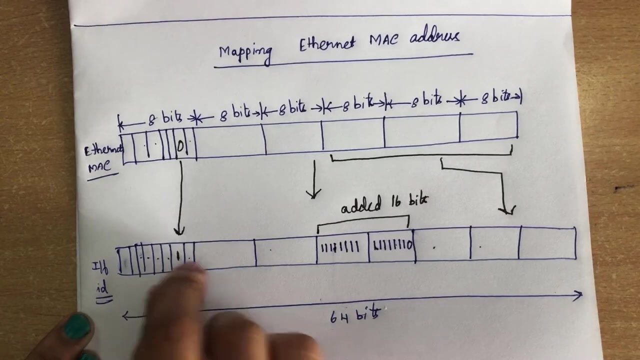 remaining bits to any site and this subnet. you can allocate to this many number of subnets. and, last is, you can allocate these many addresses inside your internet. so these are all. this is your global. this is how the address space has been divided. okay, we will see how we are going. 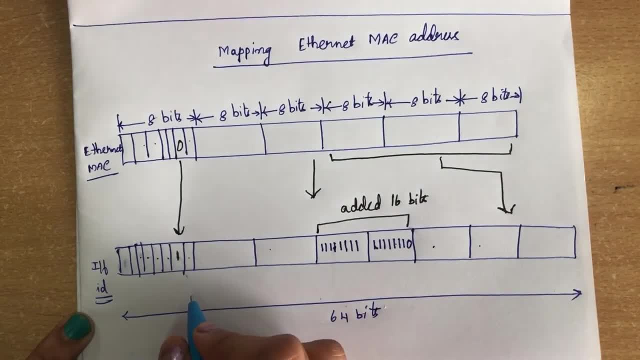 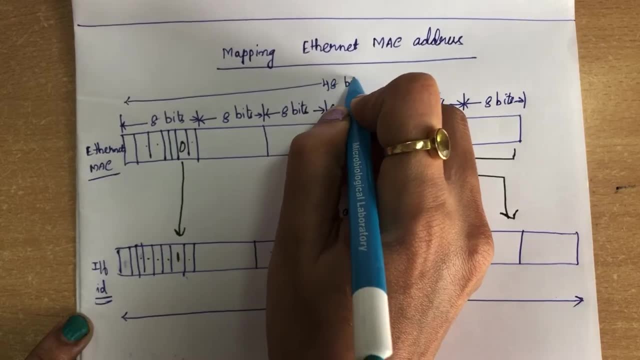 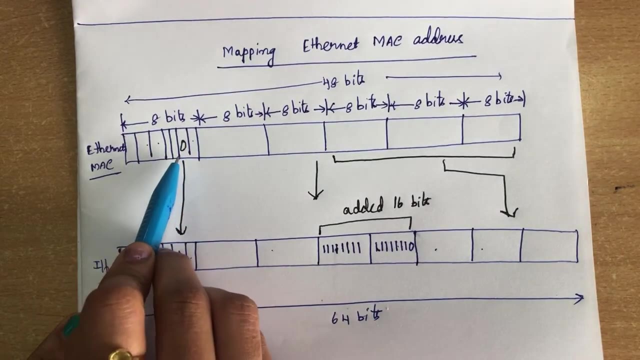 to map an ethernet address to ip version 6 address. okay, so usually this mac address is composed of 48 bits. see here it is 48 bits, which is divided into six blocks over here and the first in the first eight bits. the seventh bit is zero over here, when it is when you have your ethernet address. 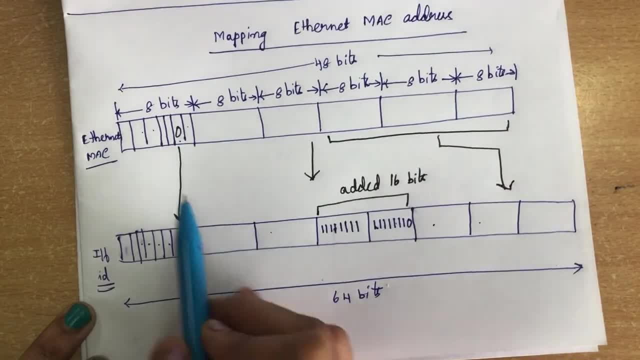 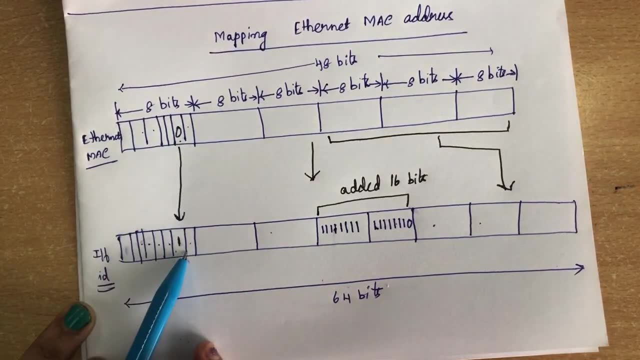 the. it will be local when you want to convert to a global one, so you need to complement the zero by one, the seventh bit of first byte. you have to convert the zero bit to one and you have to when you are going to convert this 48 bits to. 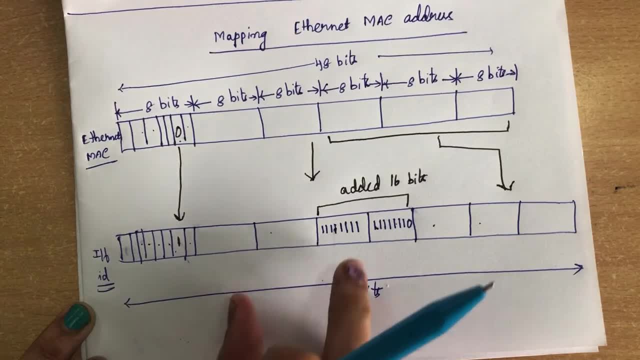 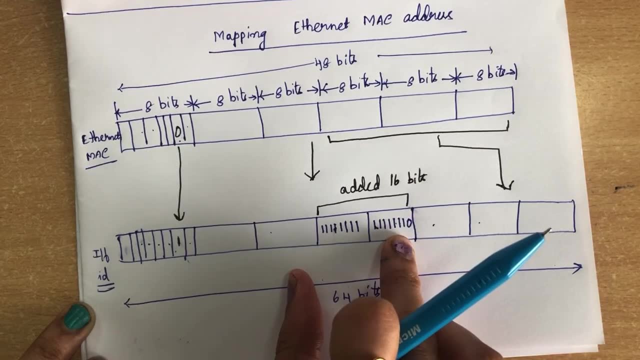 you have to convert this 48 bits to a global one, so you need to complement the zero by one 64 bits. you need to add additional 16 bits. okay, additional 16 bits, which will have the numbers, eight ones, 15 ones, followed by one zero. that additional 16 bits, it should be added after. 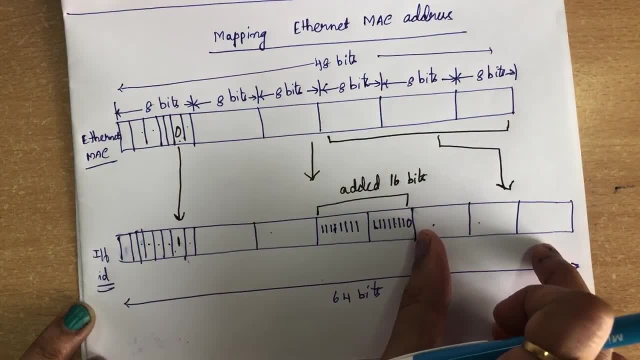 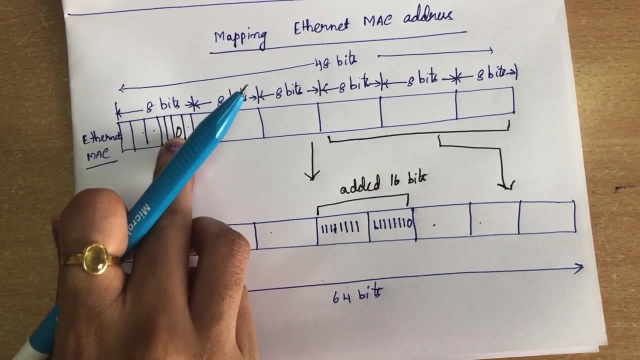 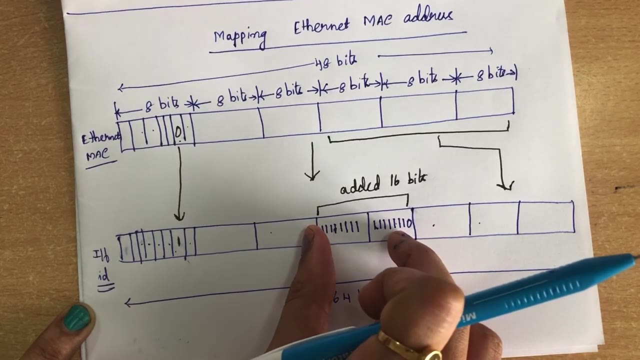 three blocks and remaining three blocks you have to take as it is so for mapping your ethernet mac address to your ip versions etc. you need to convert, complement the zero bit of first byte to one and you have to add 16 bits, of which 11 ones, that is, 15 ones, followed by one zero, which will